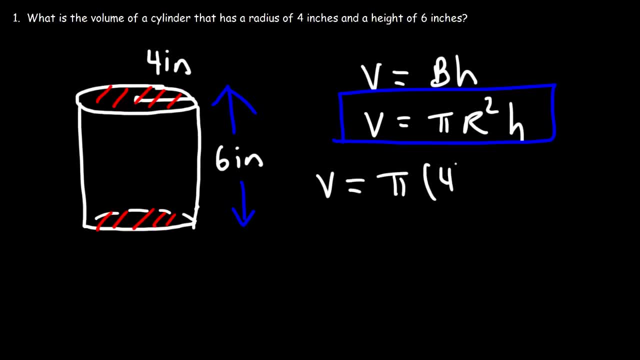 this equation. So the radius is 4 inches and the height is 6.. Now, 4 squared, that's 4 times 4, which is 16.. And 16 times 6, we know that 10 times 6 is 60.. 6 times 6 is 36.. 60 plus 36 is 96.. 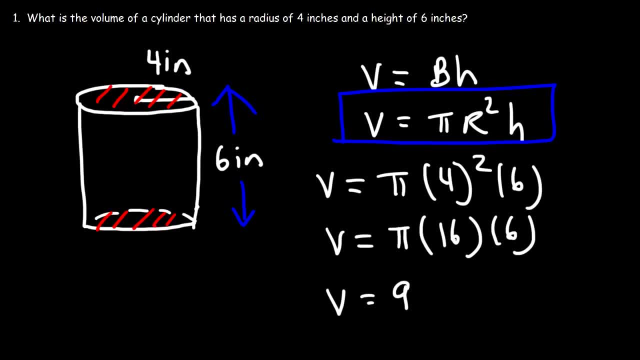 So 16 times 6 is 96.. So our answer is 96 pi cubic inches. Now, if you want to get the decimal value, here's what it's going to be. I'm going to use the pi value in my calculator. 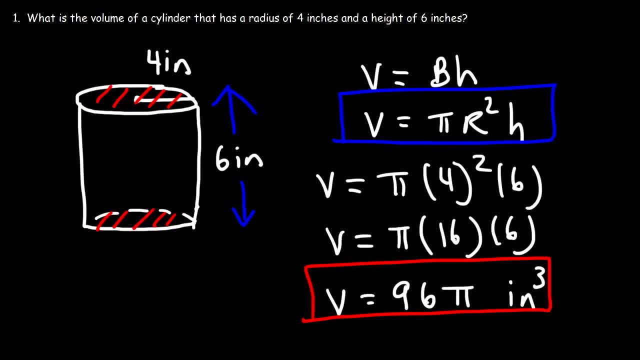 which is 3.14159, with some other numbers added to it. So let's take that, multiply it by 96.. And so I got 3.14159.. So that's 301.6 cubic inches. Now let's say, if you just use 3.14 times 96.. 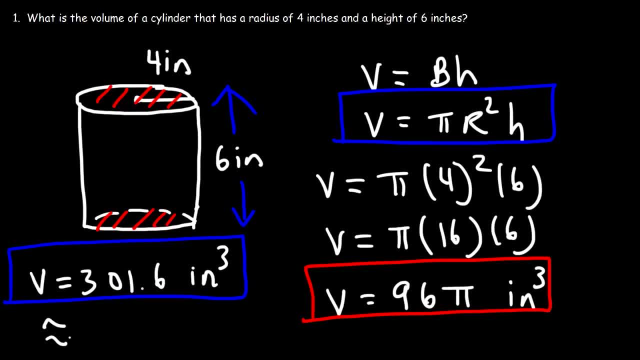 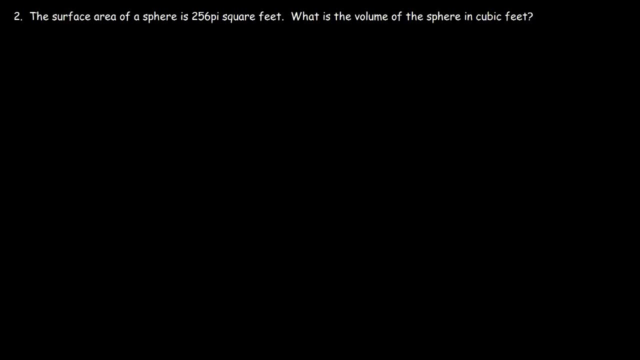 Then you should get an answer that's close to it as well: 301.44.. So depending on if you use 3.14 or a more exact value of pi, your answer will differ a little. Number two: the surface area of a sphere is 256 pi square feet. 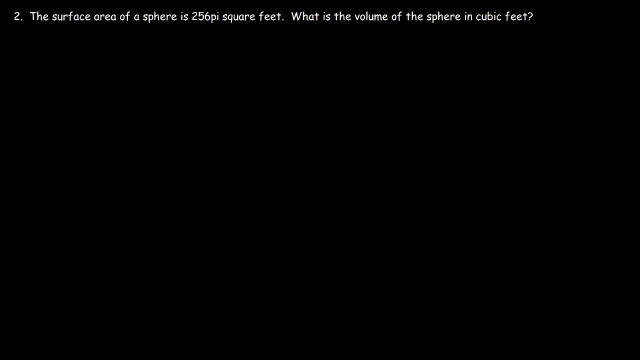 What is the volume of the sphere in cubic feet? So let's draw a picture. So this is the radius of the sphere, which is what we need to find Now the formula to calculate the volume of a sphere: it's 4 thirds pi r cubed And the surface. 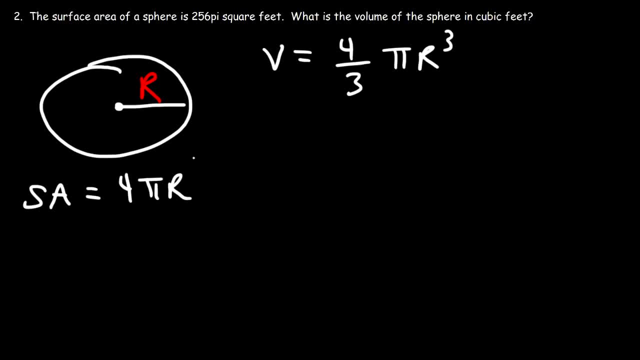 area is 4 pi r squared. So we're given the surface area and we need to calculate the radius. Once we have the radius, we can then plug it into this formula to calculate the volume. So let's go ahead and begin. 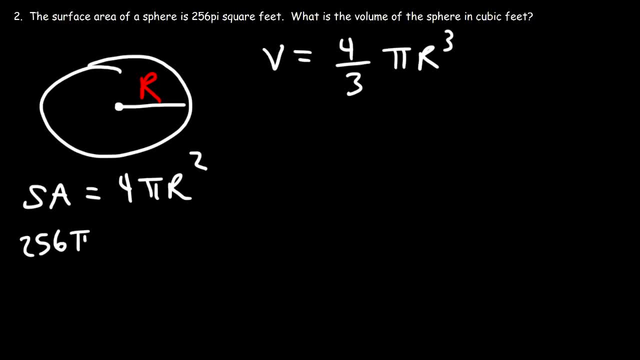 So the surface area is 256 pi And let's solve for r. So what we need to do is we need to divide both sides by 4 pi. On the right, these two will cancel. On the left, we could cancel. 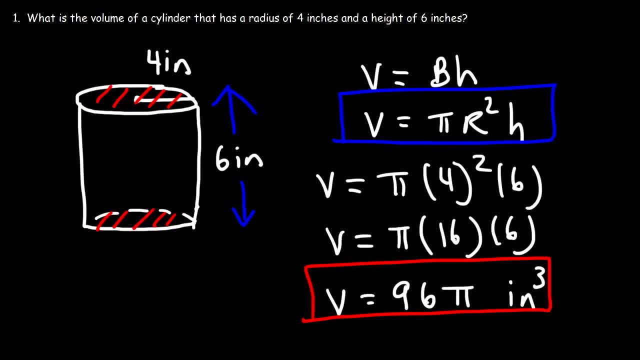 which is 3.14159, with some other numbers added to it. So let's take that, multiply it by 96.. And so I got 3.14159.. So that's 301.6 cubic inches. Now let's say, if you just use 3.14 times 96.. 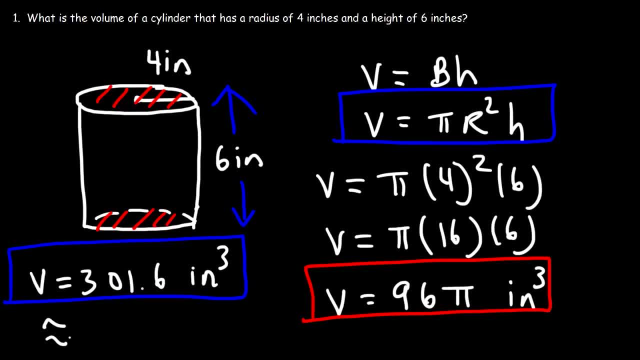 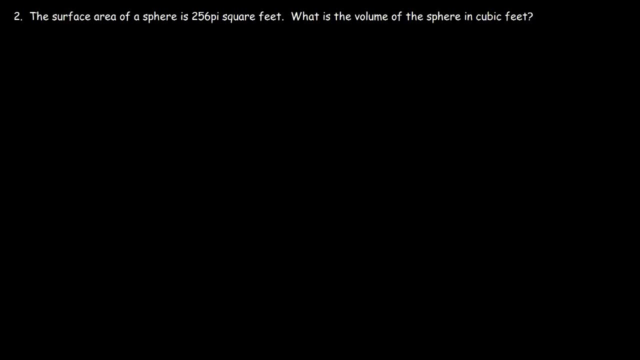 Then you should get an answer that's close to it as well: 301.44.. So depending on if you use 3.14 or a more exact value of pi, your answer will differ a little. Number two: the surface area of a sphere is 256 pi square feet. 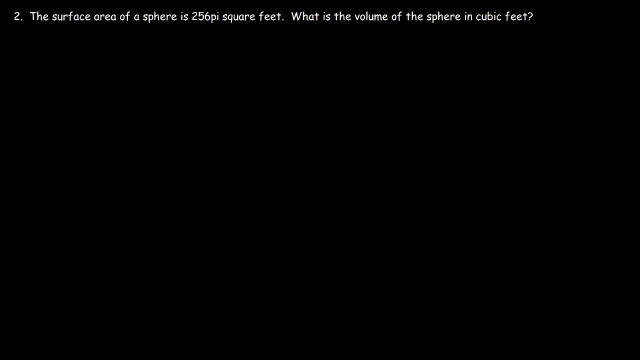 What is the volume of the sphere in cubic feet? So let's draw a picture. So this is the radius of the sphere, which is what we need to find Now the formula to calculate the volume of a sphere: it's 4 thirds pi r cubed And the surface. 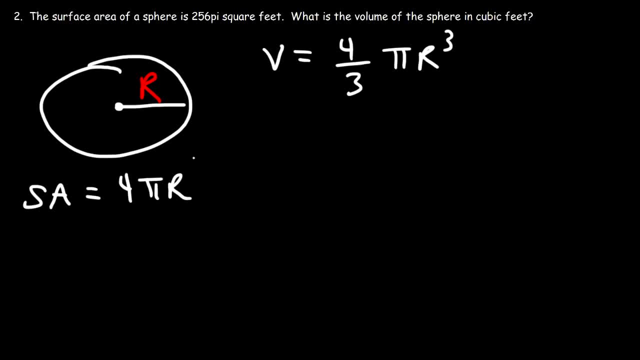 area is 4 pi r squared. So we're given the surface area and we need to calculate the radius. Once we have the radius, we can then plug it into this formula to calculate the volume. So let's go ahead and begin. 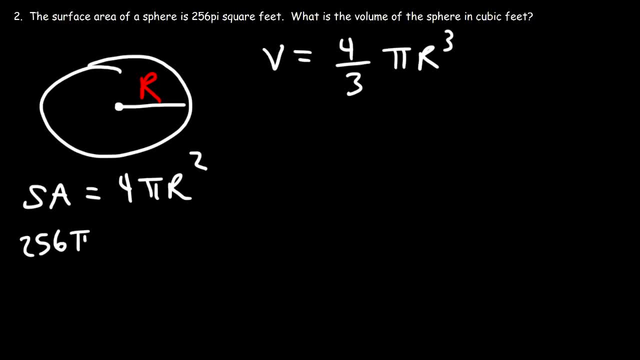 So the surface area is 256 pi And let's solve for r. So what we need to do is we need to divide both sides by 4 pi. On the right, these two will cancel. On the left, we could cancel. 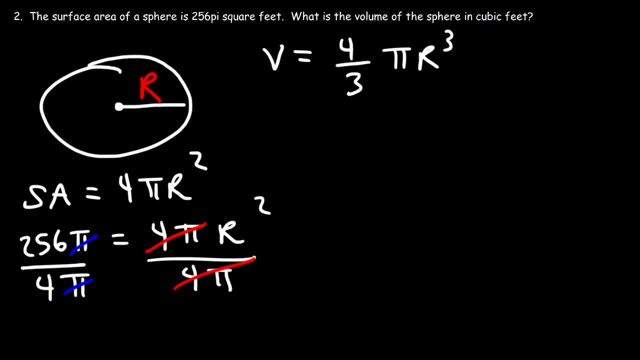 And so 256 divided by 4 is 64.. So we have: 64 is equal to r squared, And now we can take the square root of both sides. So the square root of 64 is 8.. So the radius is 8 feet. 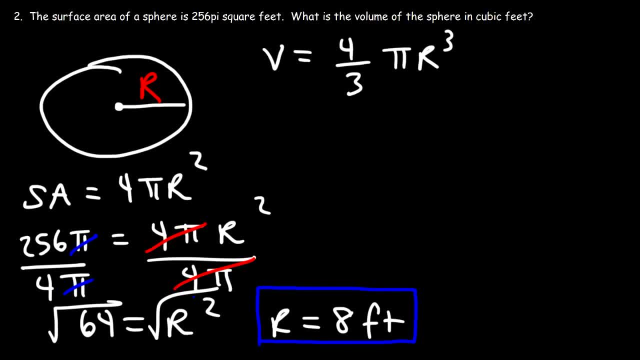 So now that we have the radius, we can now calculate the volume. So the volume is going to be 4 over 3 pi times r cubed, But r is 8.. So 8 raised to the third power, That's 8 times 8 times 8.. 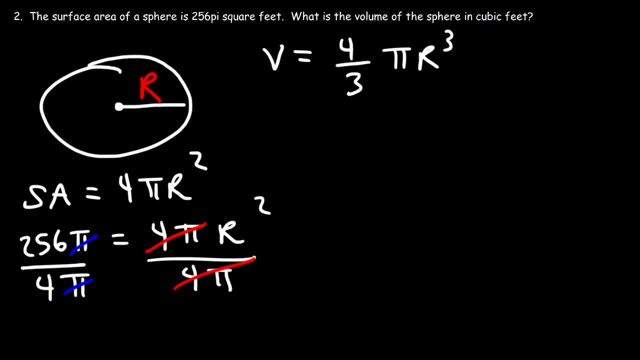 And so 256 divided by 4 is 64.. So we have: 64 is equal to r squared, And now we can take the square root of both sides. So the square root of 64 is 8.. So the radius is 8 feet. 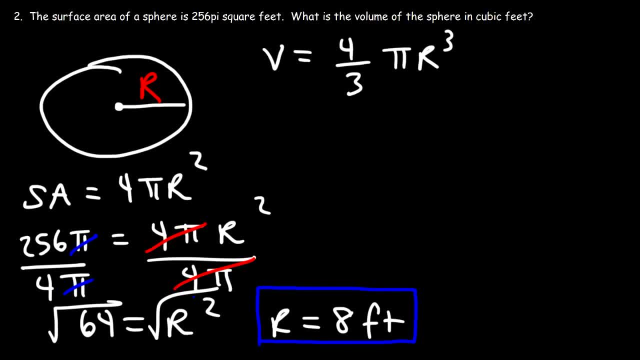 So now that we have the radius, we can now calculate the volume. So the volume is going to be 4 over 3 pi times r cubed, But r is 8.. So 8 raised to the third power, That's 8 times 8 times 8.. 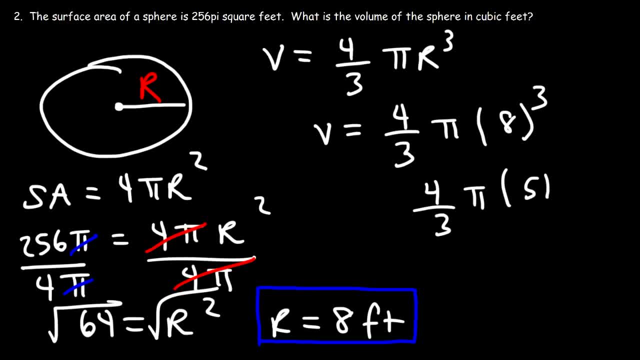 And so that's going to be 512.. So 512 times 4 divided by 3.. So that's 2048 over 3 times pi. So this is our answer. in cubic feet That's the exact answer: 2048 pi over 3.. 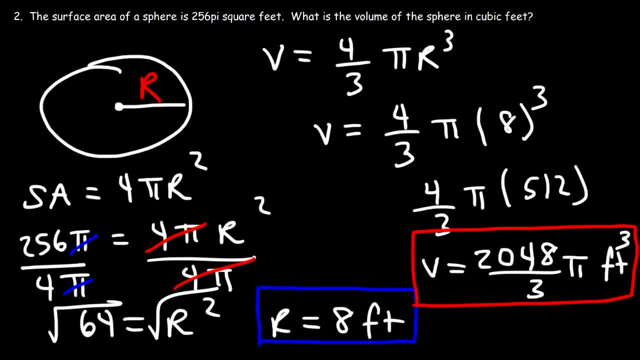 Now to get the decimal value, let's multiply pi, which is 3.14159 times 2048 divided by 3. And so you should get 2144.66,, but I'm going to round it to 0.7.. 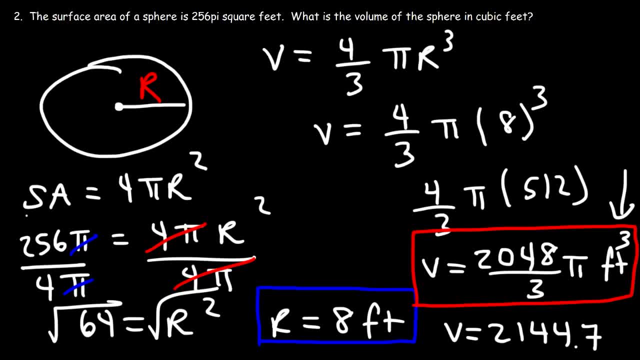 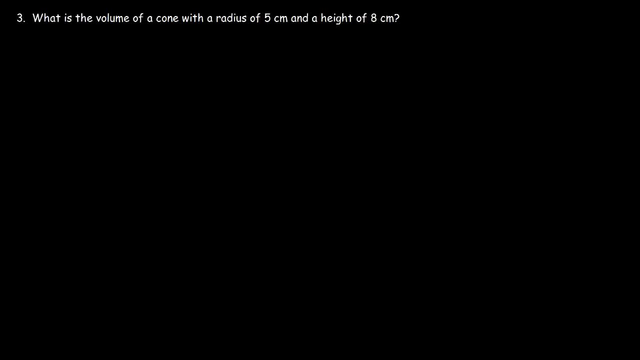 And the unit's cubic feet. And so that's the volume of this sphere. That's how you could find it if you're given the surface area of a sphere. Now let's move on to the third question. What is the volume of a cone with a radius of 5 centimeters and a height of 8 centimeters? 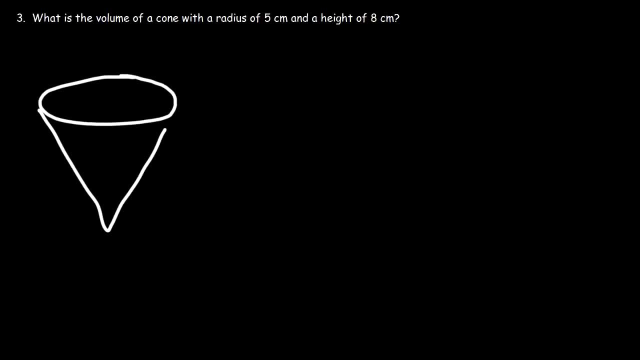 So let's begin with a picture. So here we have a cone, And here the radius is 5 centimeters, And then the height, which is basically 8 centimeters. It's this distance, It's here. So, with this information, given the radius and the height, 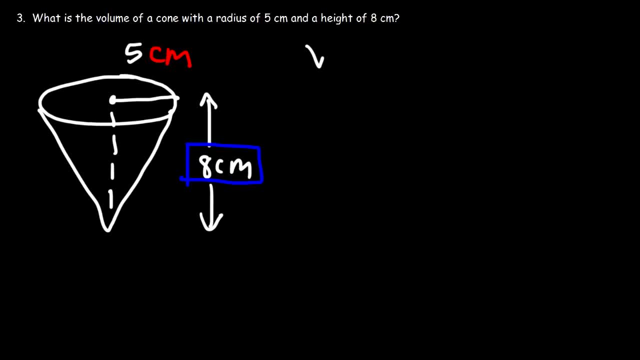 what is the volume of the cone? All we need to do is use this formula: The volume of a cone is 1 third of that of a cylinder, So it's 1 third pi r squared times the height. So we have the radius, which is 5.. 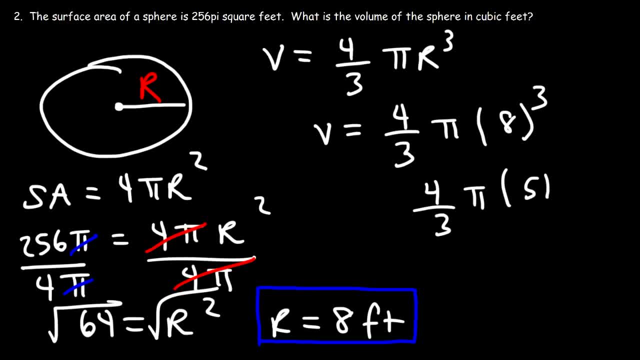 And so that's going to be 512.. So 512 times 4 divided by 3.. So that's 2048 over 3 times pi. So this is our answer. in cubic feet That's the exact answer: 2048 pi over 3.. 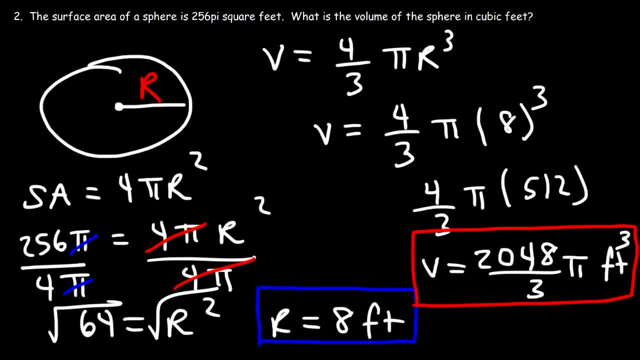 Now to get the decimal value, let's multiply pi, which is 3.14159 times 2048 divided by 3. And so you should get 2144.66,, but I'm going to round it to 0.7.. 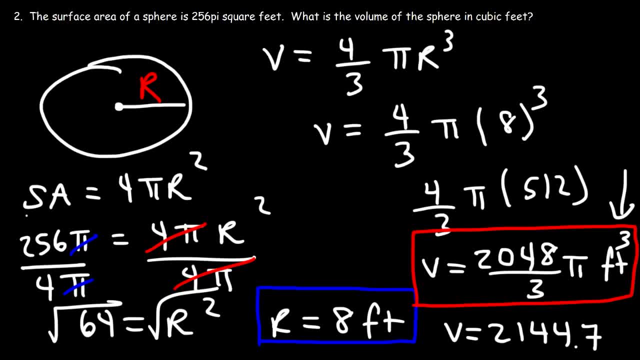 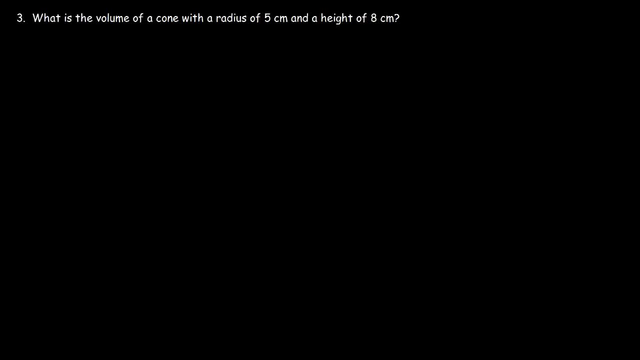 And the unit's cubic feet. And so that's the volume of this sphere. That's how you could find it if you're given the surface area of a sphere. Now let's move on to the third question. What is the volume of a cone with a radius of 5 centimeters and a height of 8 centimeters? 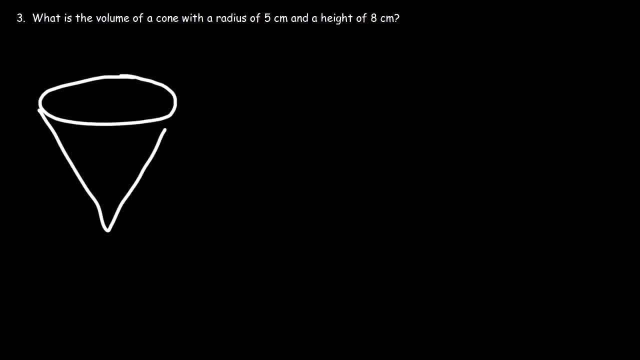 So let's begin with a picture. So here we have a cone, And here the radius is 5 centimeters, And then the height, which is basically 8 centimeters. It's this distance And then the height, which is this distance here. 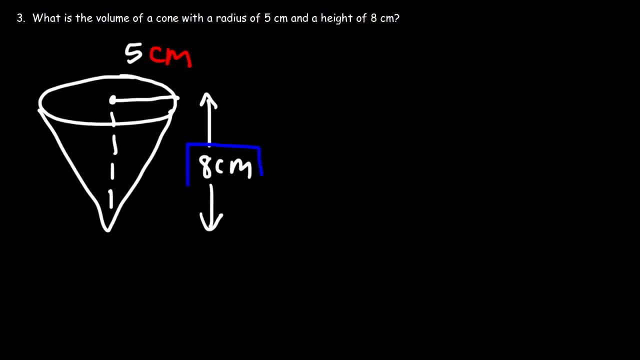 So, with this information, given the radius and the height, what is the volume of the cone? All we need to do is use this formula: The volume of a cone is 1 third of that of a cylinder, So it's 1 third pi r squared times the height. 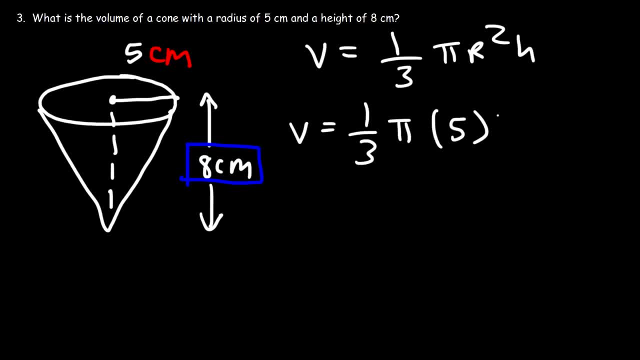 So we have the radius, which is 5.. And we know the height, which is 8.. 5 squared, or 5 times 5, is 25.. And what is 25 times 8?? So we have the radius, which is 5.. 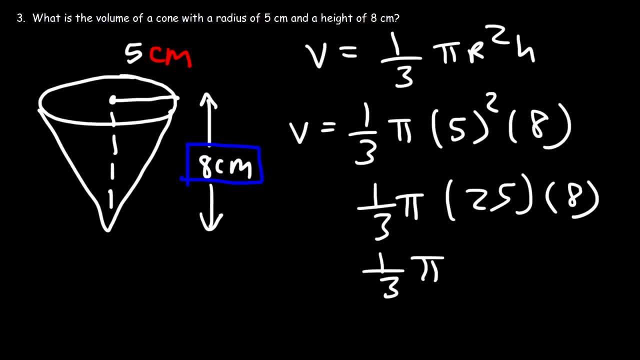 So if you had 8 quarters, how much money do you have? 8 quarters is basically $2.. So 25 times 8 is 200. And so our answer is going to be 200 pi over 3.. And we're dealing with centimeters. 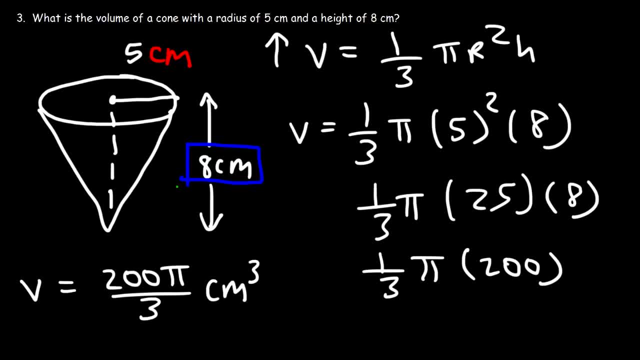 And so this is going to be cubic centimeters. The units for volume is always cubic units, Cubic centimeters, cubic feet, cubic inches or something like that. So now let's convert this into a decimal, So 200 pi divided by 3.. 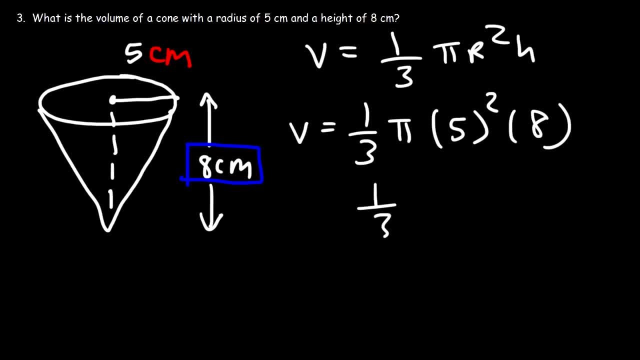 And we know the height, which is 8.. 5 squared, or 5 times 5, is 25.. And what is 25 times 8?? So we have the radius, which is 5.. So if you had 8 quarters, how much money do you have? 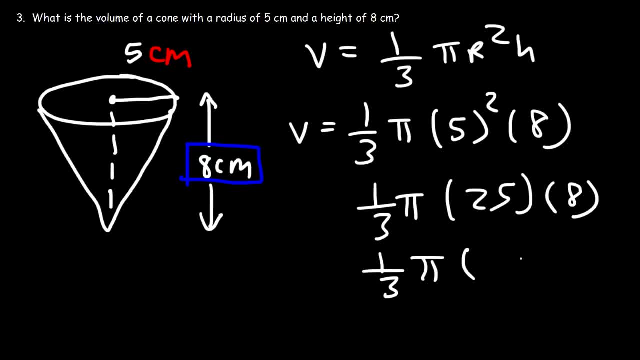 8 quarters is basically $2.. So 25 times 8 is 200. And so our answer is going to be 200 pi over 3. And we're dealing with centimeters, And so this is going to be cubic centimeters. 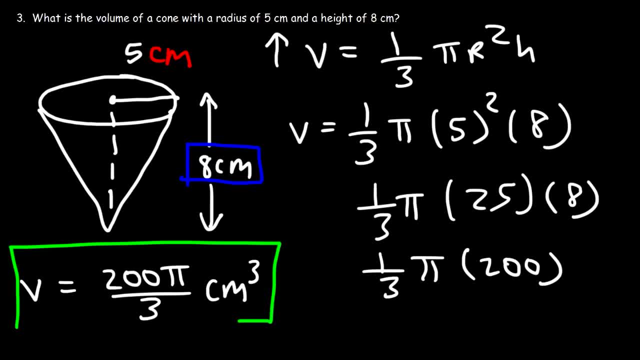 The units for volume is always cubic units: Cubic centimeters, cubic feet, cubic inches or something like that. So now let's convert this into a decimal. So 200 pi divided by 3. Is the same as 209.44, if you round it. cubic centimeters. 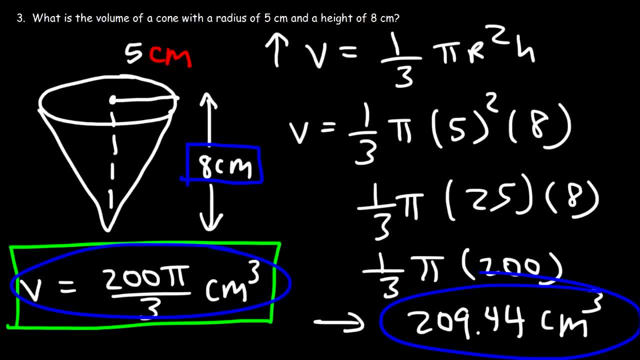 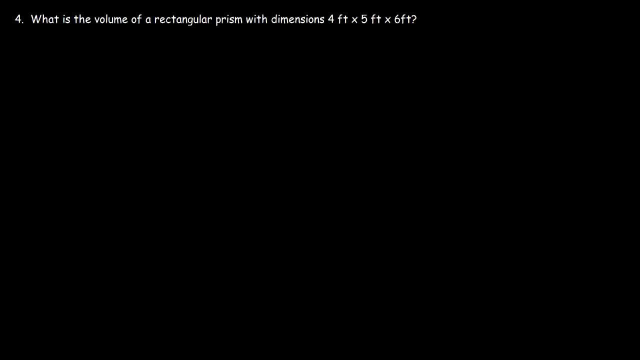 And so you can report your answer like this, if you want to, or like this Number 4.. What is the volume of a rectangular prism with dimensions 4 feet by 5 feet by 6 feet? So here's a rectangular prism. 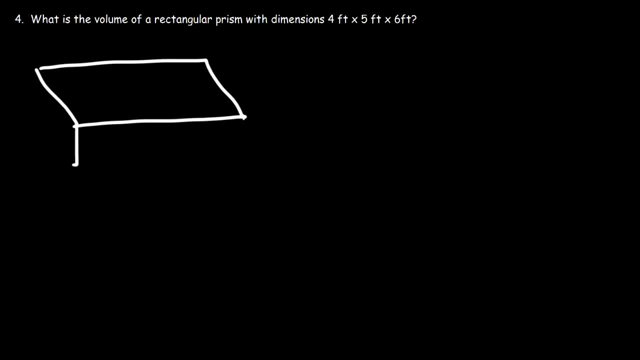 It looks like a box, And so that's how we can draw it. To find the volume, you just need to multiply the length by the width, by the height, And so this problem is not going to be too difficult, Because we have the length and the width and the height. 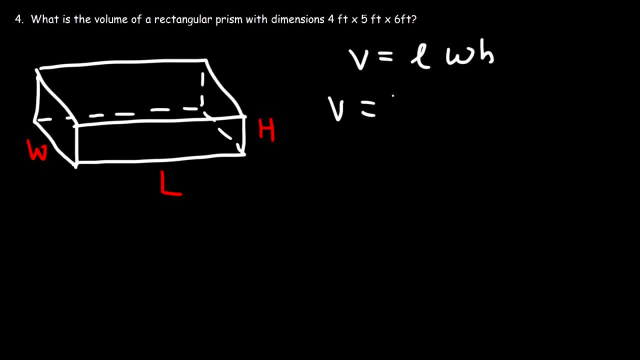 It really doesn't matter. It really doesn't matter what order we multiply those three numbers. So it's just going to be 4 feet times 5, feet times 6 feet, And 4 times 5 is 20.. And 20 times 6.. 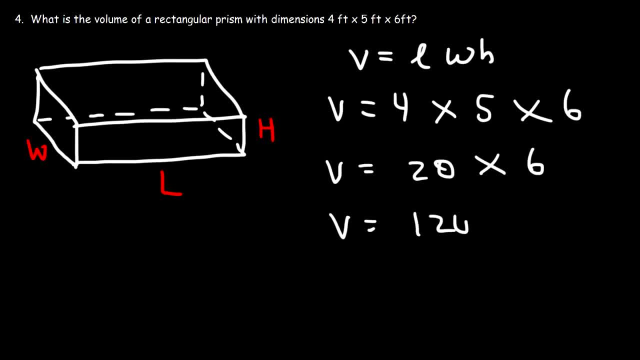 If you have 6 $20 bills, you have $120. And since we multiplied feet by feet by feet, it's going to be cubic feet, Or feet raised to the third power, And so that's the volume of this particular rectangular prism. 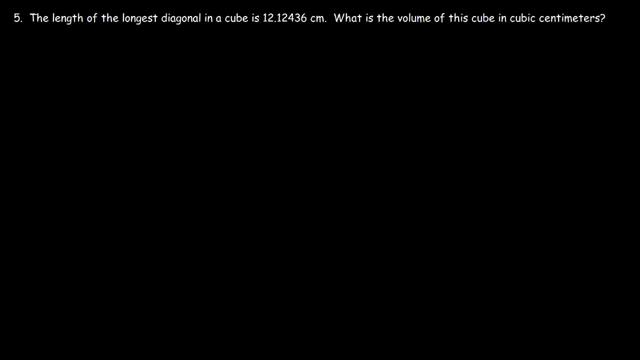 What about this problem? The length of the longest diagonal in the cube is 12.12436 centimeters. What is the volume of this cube in cubic centimeters? So if we're given the diagonal length of a cube, the longest diagonal, 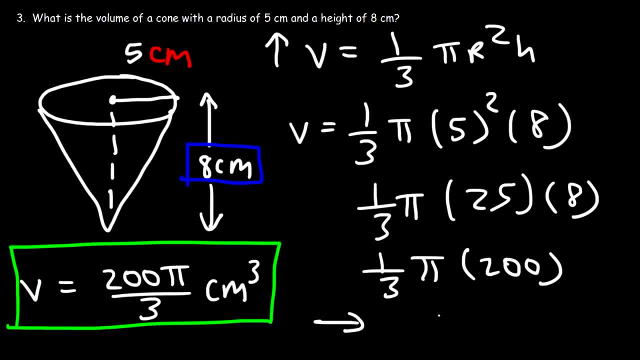 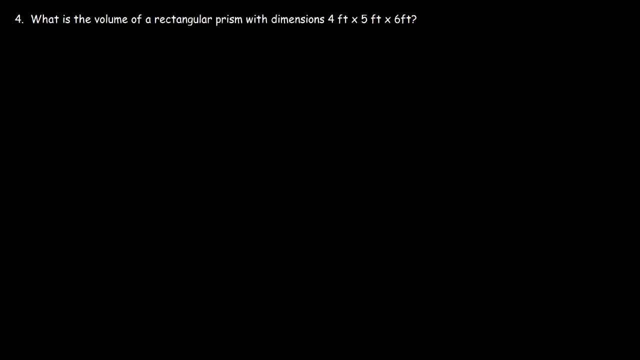 Is the same as 209.44, if you round it cubic centimeters, And so you can report your answer like this, if you want to, or like this Number 4.. What is the volume of a rectangular prism with dimensions 4 feet by 5 feet by 6 feet? 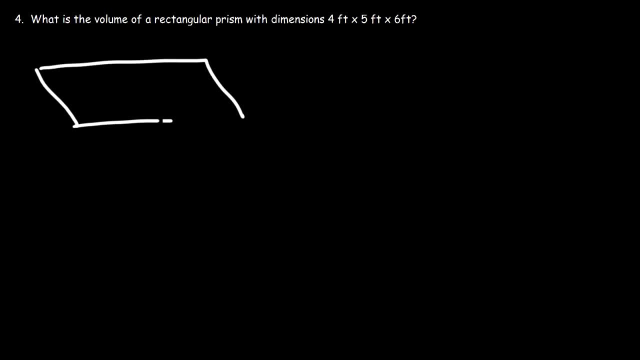 So here's a rectangular prism. It looks like a box, And so that's how we can draw it. To find the volume, you just need to multiply the length by the width, by the height, And so this problem is not going to be too difficult. 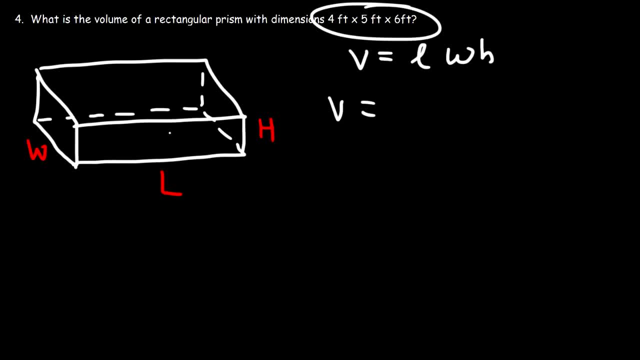 Because we have the length and the width and the height. So we're going to multiply the length by the width, by the height. It really doesn't matter what order We multiply those three numbers, So it's just going to be 4 feet times 5 feet times 6 feet. 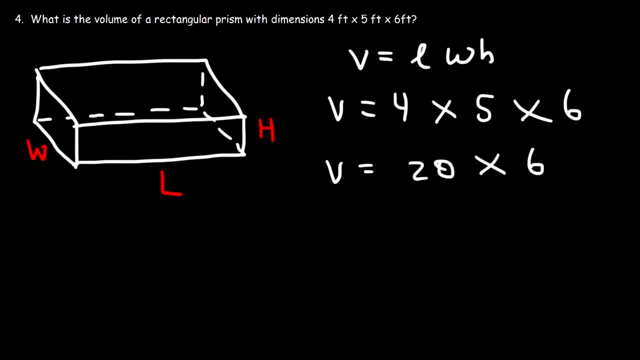 And 4 times 5 is 20.. And 20 times 6. If you have 6 $20 bills, you have $120. And since we multiplied feet by feet by feet, it's going to be cubic feet, Or feet raised to the third power. 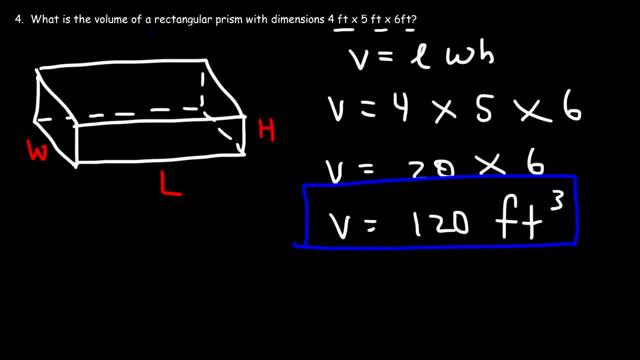 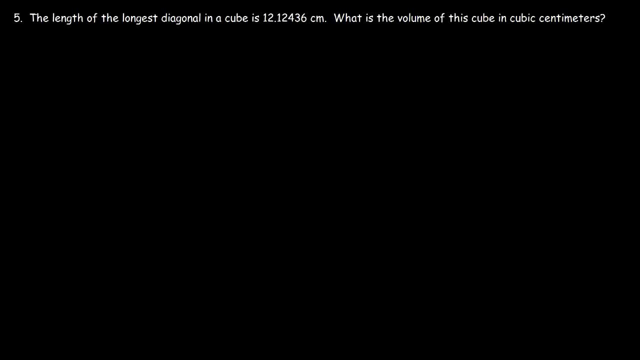 And so that's the volume of this particular rectangular prism. What about this problem? The length of the longest diagonal in the cube is 12.12436 centimeters. What is the volume of this cube in cubic centimeters? So if we're given the diagonal length of a cube, the longest diagonal 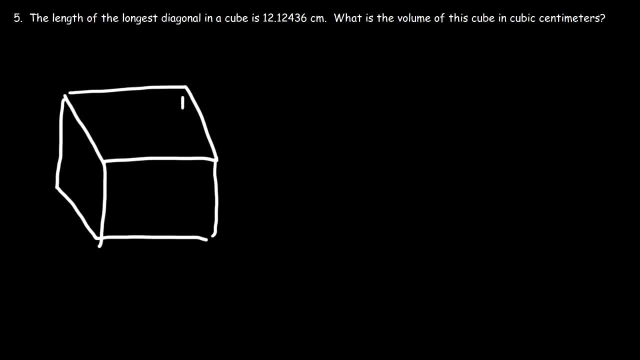 how can we use that to calculate the volume of a cube? So let's call this point A, B and C. So the distance between A and B, that's one diagonal And the distance between A and C is the longest diagonal, which is what we're trying to find. 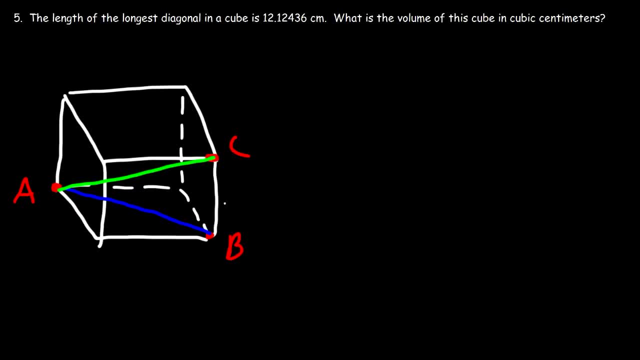 Now for a cube. all sides are the same, So we can call this X, X and X. So if we focus on, let's say, the blue triangle, Notice that we can come up with this equation. Let's call the hypotenuse of that triangle L. 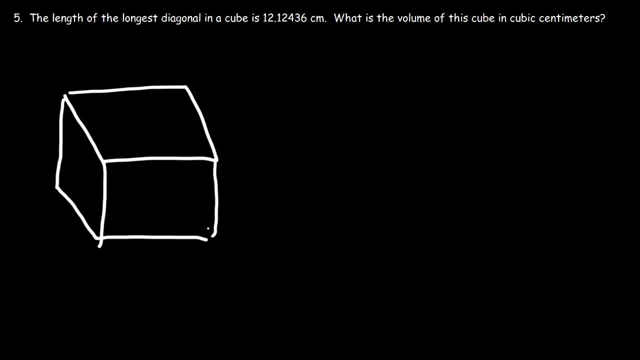 how can we use that to calculate the volume of a cube? So let's call this point A, B and C. So the distance between A and B, that's one diagonal And the distance between A and C is the longest diagonal, which is what we're trying to find. 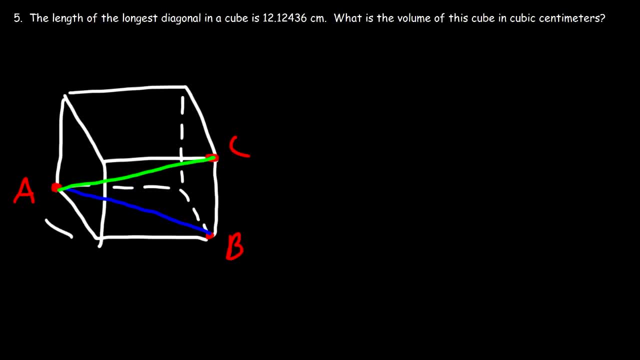 Now for a cube. all sides are the same, So we can call this X, X and X. So if we focus on, let's say, the blue triangle, Notice that the blue triangle is the longest diagonal, Notice that we can come up with this equation. 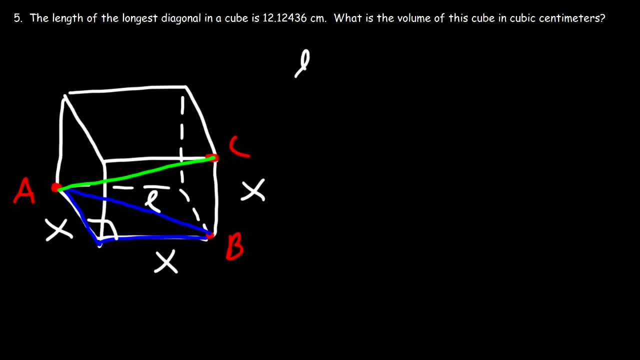 Let's call the hypotenuse of that triangle L. So L squared is equal to X squared plus X squared. Now if we focus on, let's say, the green triangle- Let me draw that better- Notice that we can use the Pythagorean theorem again. 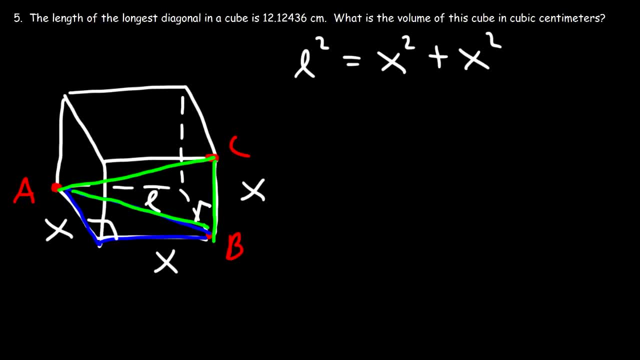 which is A squared plus B squared, equals C squared. But here we have L and X And let's call The longest diagonal D, which is what we're trying to find. Let me use a different color for that, So we can say that D squared. the hypotenuse for the green triangle. 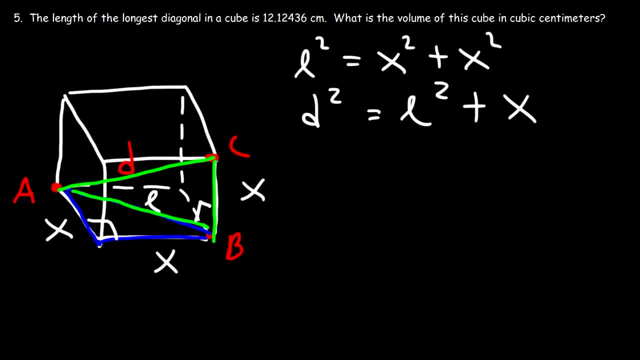 is L squared plus X squared. So now, because L squared is X squared plus X squared, I'm going to replace L squared in the second equation. So I have: D squared is X squared plus X squared plus another X squared, So D squared is equal to. 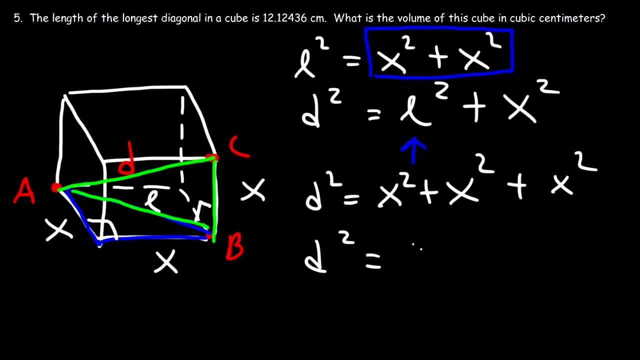 1X squared plus 1X squared plus 1X squared is 3X squared. Now, if we take the square root of both sides, the length of the diagonal of a cube is the square root of 3 times the side length. 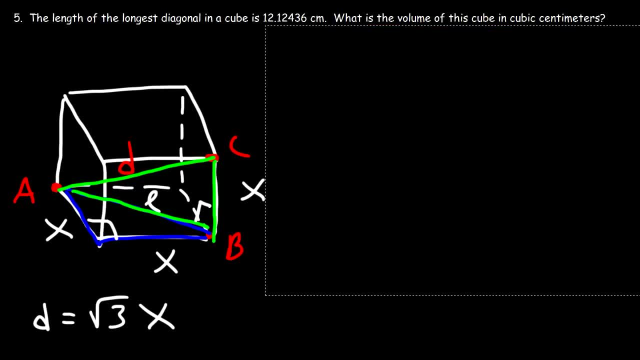 And so that's the formula that we need in this example. Now, we mentioned that the volume of a rectangular prism is the length times the width times the height. In this case, for the cube, the length and the width and the height are the same. 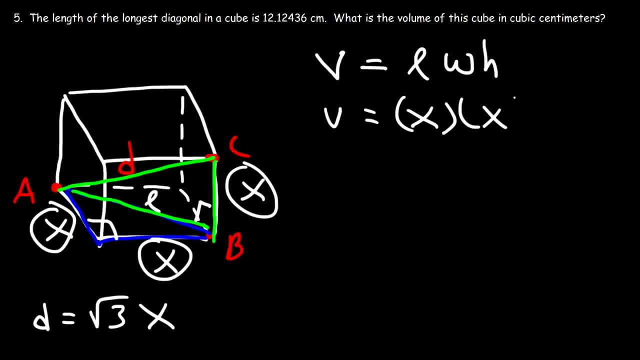 For the height they're all X. So X times X times X. So the volume of a cube is X cubed. So let's write that equation here and we're going to use it later. So first we need to calculate X using this formula: 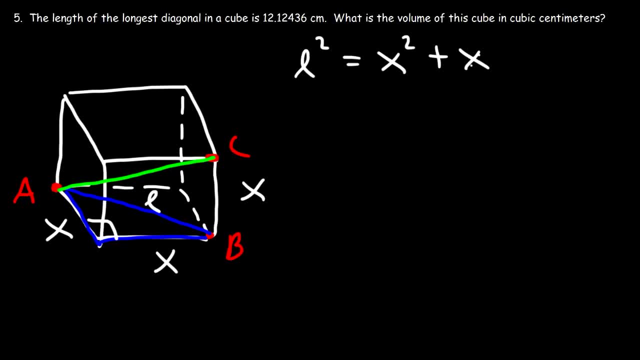 So L squared is equal to X squared plus X squared. Now, if we focus on, let's say, the green triangle- Let me draw that better- Notice that we can use the Pythagorean theorem again, which is: A squared plus B squared equals C squared. 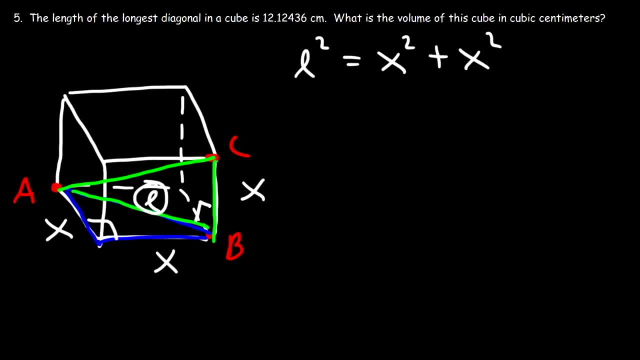 But here we have L and X And let's call the longest diagonal D, which is what we're trying to find. But let me use a different color for that, So we could say that D squared the hypotenuse for the green triangle. 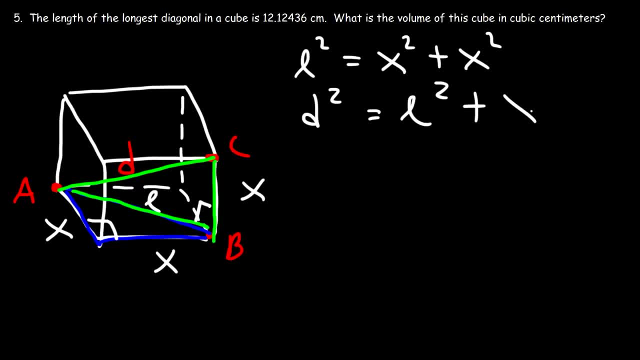 is L squared plus X squared. So now, because L squared is X squared plus X squared, I'm going to replace L squared in the second equation. So I have: D squared is X squared plus X squared, plus another X squared. So D squared is X squared plus X squared plus another X squared. 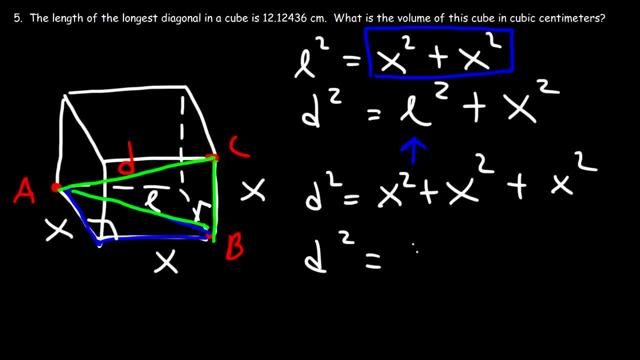 So D squared is equal to 1X squared plus 1X squared plus 1X squared is 3X squared. Now, if we take the square root of both sides, the length of the diagonal of a cube is the square root of 3 times the side length. 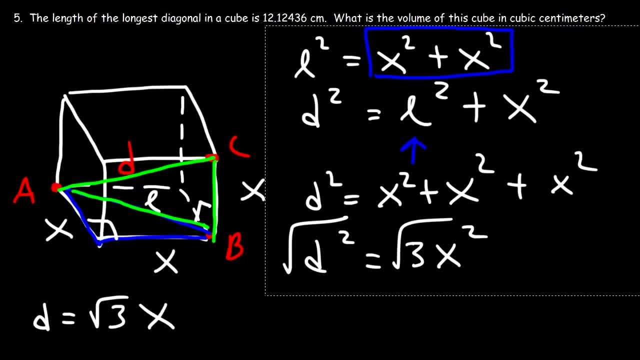 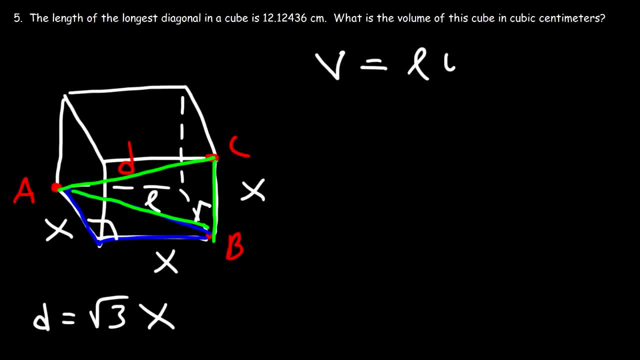 And so that's the formula that we need in this example. Now, we mentioned that the volume of a rectangular prism is the length times the width times the height. In this case for the cube, the length and the width and the height. 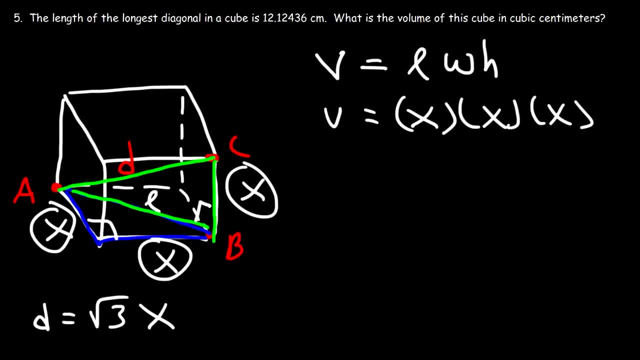 they're all X. So X times X times X. So the volume of a cube is X cubed. So let's write that equation here and we're going to use it later. So first we need to calculate X using this formula. 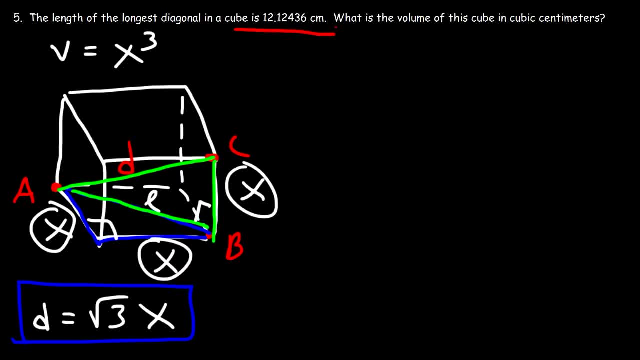 And so we have the length of the diagonal, which is 12.12436 centimeters, And that's equal to the square root of 3 times X. So let's divide both sides by the square root of 3.. If you divide 12.12436 by the square root of 3,, 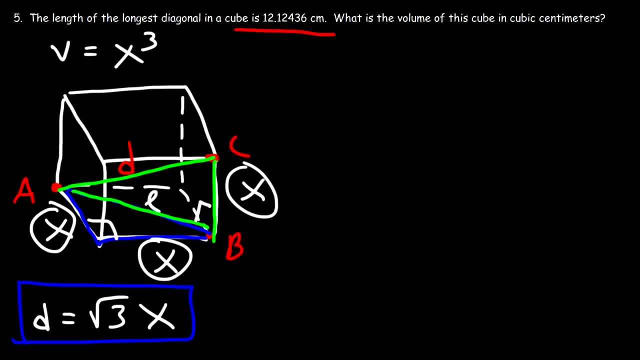 And so we have the length of the diagonal, which is 12.12436 centimeters, And that's equal to the square root of the diagonal, which is the square root of 3 times X. So let's divide both sides by the square root of 3.. 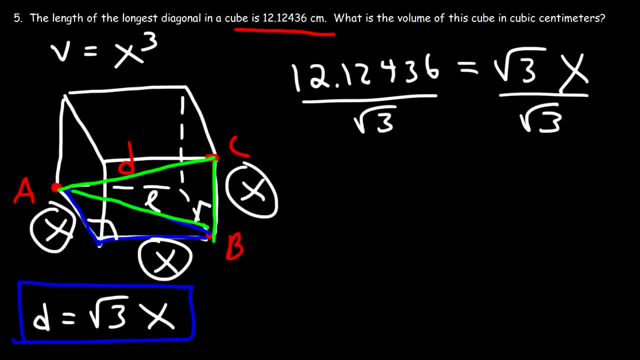 If you divide 12.12436 by the square root of 3, you get 7.. Technically it's like 7.0000251, but for the most part that's about 7.. So X is 7.. 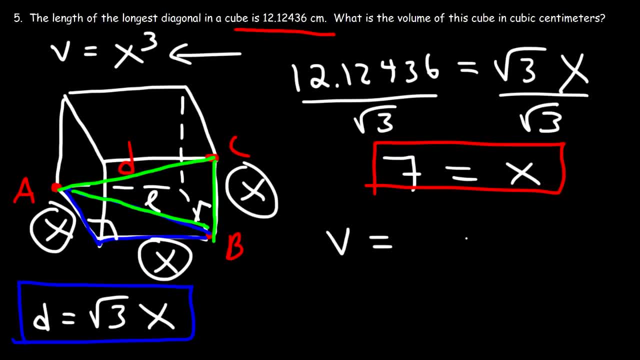 Now we can use this equation. So the volume is going to be 7 centimeters raised to the 3rd power. So 7 to the 3rd power, or 7 times 7 times 7, that's 343.. 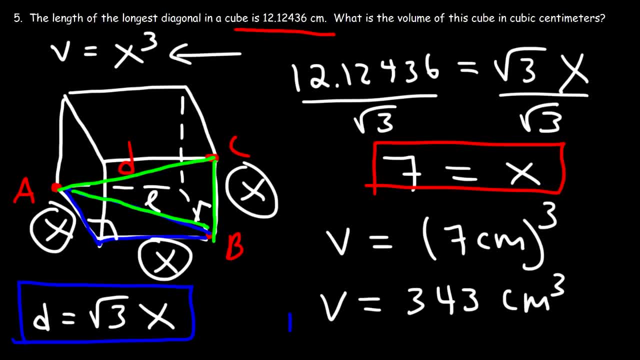 So our final answer is 343 cubic centimeters, And so now you know how to find the volume of common shapes like cubes, rectangular prisms, cones, cylinders and spheres, And so that's it for this video. Thanks for watching. See you next time. 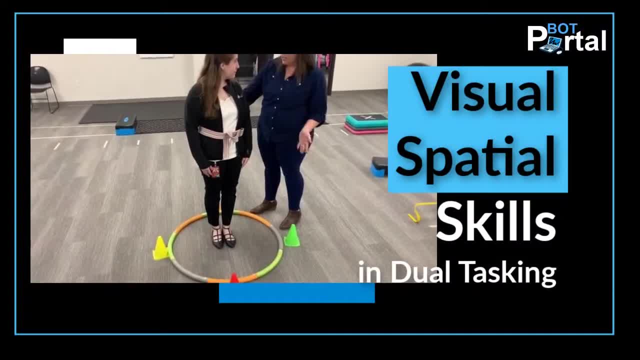 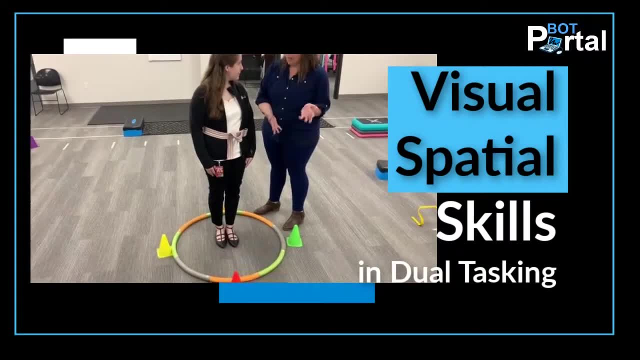 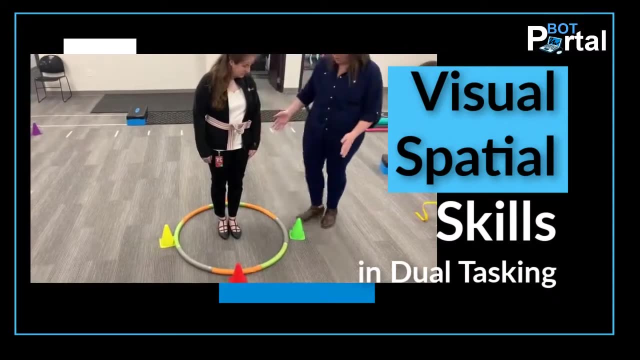 Okay, Jenna, so today we're going to be doing a activity that's going to test your balance and we're going to work on that, but we're also going to be working on your ability to tell time and figure out where it is in space. Okay, so if you'll take a look at the ground, 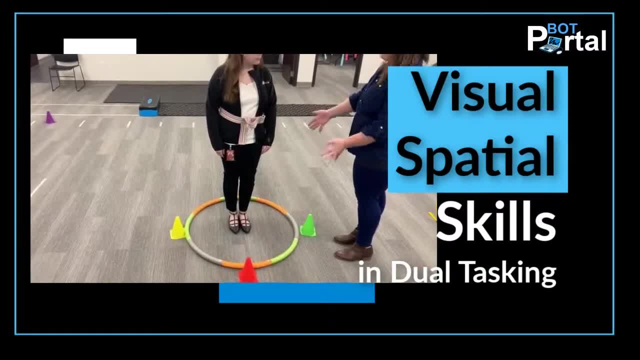 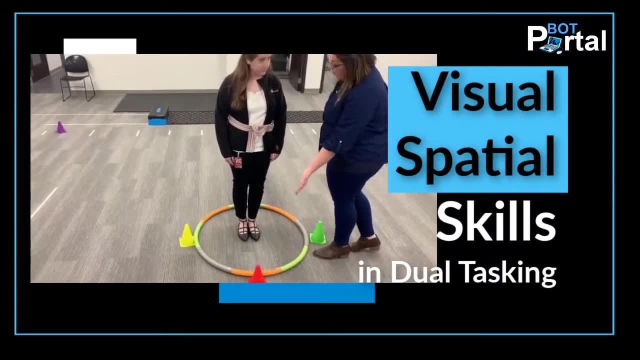 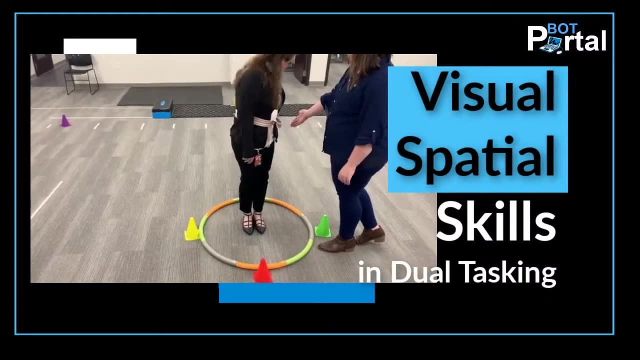 we have four cones. You are in the face of a clock right now, so you are directly in the middle of a clock. We have the red cone, which, if you were in a clock, what time would that be? 12. Perfect. The orange cone would be Six. The yellow cone Three.